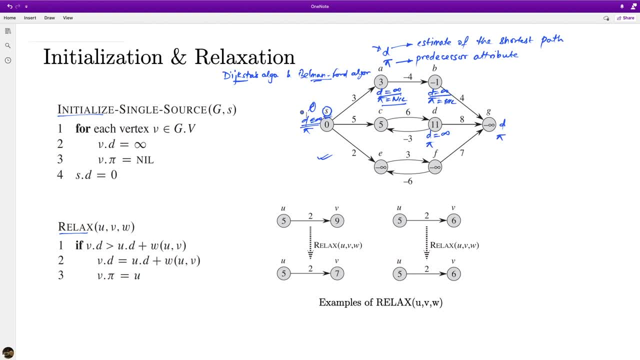 because the cost of going from the starting node to the starting node itself is zero. So this is done in this for loop. So for each vertex, all I'm doing is setting the D attribute to infinite and the pi attribute to null And finally I'm setting the D attribute for my vertex. 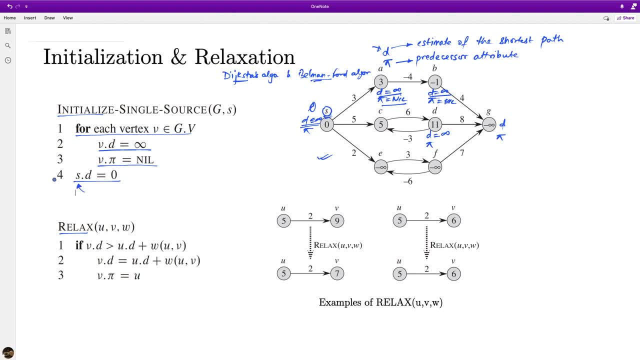 So this is for each vertex. All I'm doing is setting the D attribute to infinite and the pi attribute to null, my starting node, starting vertex, to zero. So this process simply takes my graph G, which is simply my vertices and edges, and then this is starting vertex S, and then performs these: 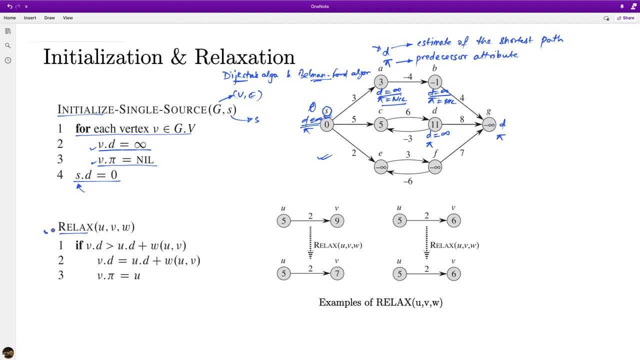 initializations to all the vertices in my graph. Next is the relax operation. So the relax operation takes two vertices, U and V, and also all the set of possible weights. So this can be a weight matrix or just the weight between U and V, and what it does is relaxes this vertex V by considering the shortest path estimate. 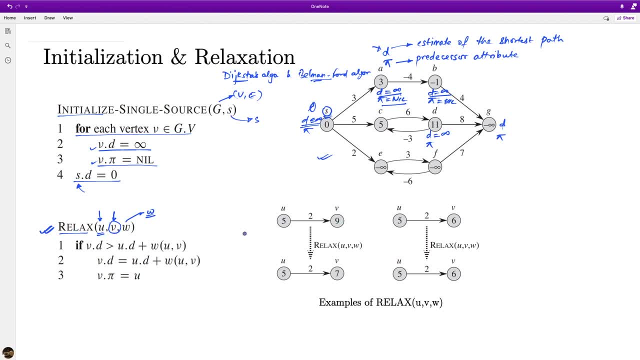 of the vertex U. So say we have a part of the graph that looks like this and say: because of some operation we found out that the shortest path estimate to U is 5, and now we know that there is a path from U to V that costs 2.. So this means that, and also let's say that 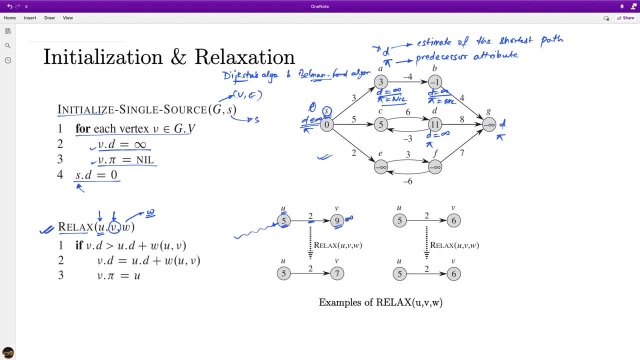 V already has a shortest path estimate of 9,. this could be infinite or this could be some any value that is appropriate for V. Now that we have found the shortest path estimate of U to be 5, we know that if we take this path of 5 plus 2, then we can reach to V with 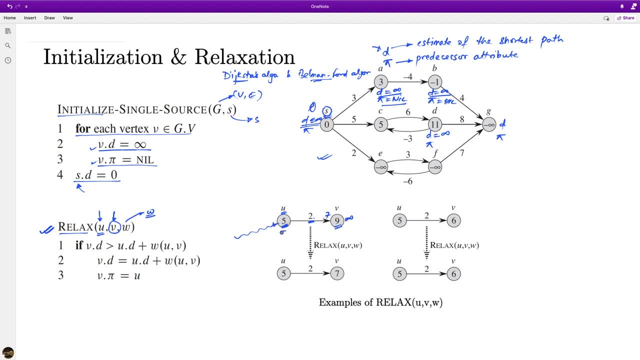 a cost of 7.. This process of looking at the shortest path estimate of a node that connects to my node V from U to V and updating the shortest path estimate for my node V by looking at the shortest path estimate of my previous node is what the relax operation does. So 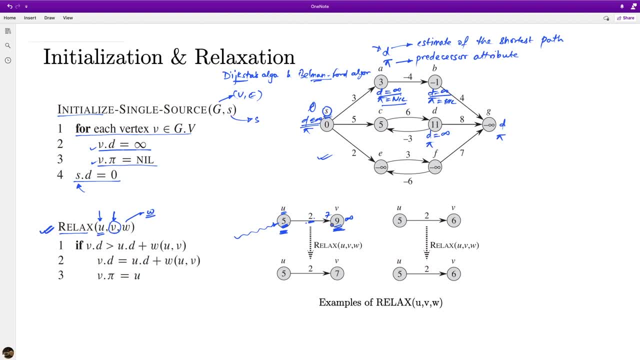 here: 5 plus 2 is 7. so my V shortest path estimate for V updates from 9 to 7.. Now what if V already has a really good shortest path estimate? So say, we have a situation like this where we at some point ended up updating the shortest path estimate for U to V, 5 and